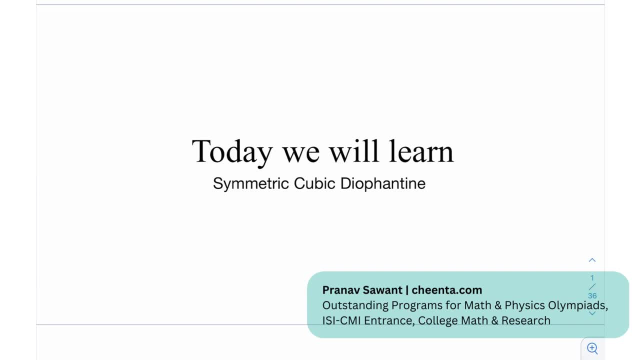 Hi everyone. So today I have with you a very beautiful problem. So this is a simple. it's one of the most classic number theory problems out there And this is a rather famous problem. So you might have seen a problem, you might have seen this problem or you might have seen some. 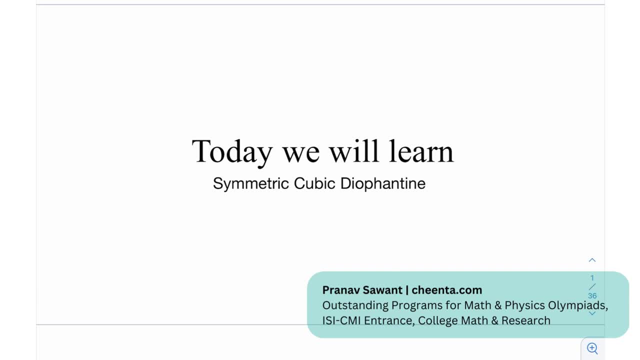 similar problems. A lot of iterations have been made to this question to make it a little bit more challenging, a little bit more interesting, But I think for anybody who is starting out with number theory, this is a very, very good introduction to this And I think this covers. 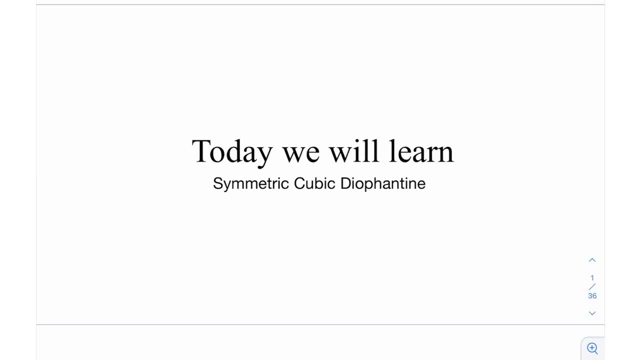 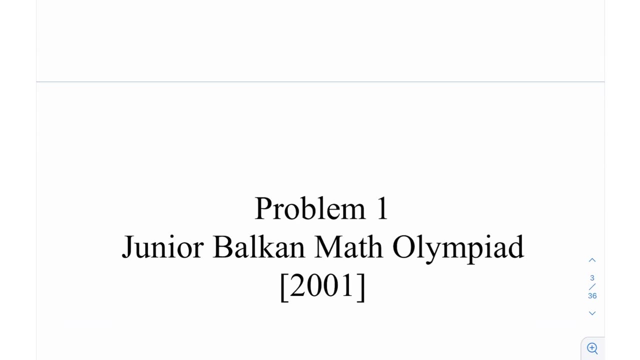 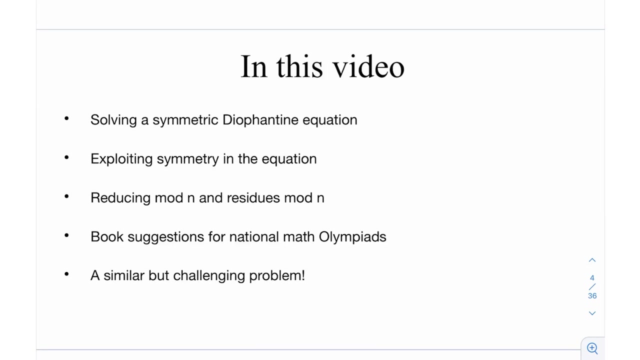 up quite a bit of areas of elementary number theory. So, without wasting any time, let's just get right into it. So this is a problem number one from the junior biopharmacologist JB Emo, back in the year 2001.. And in this video we're going to be seeing how we can solve a symmetric 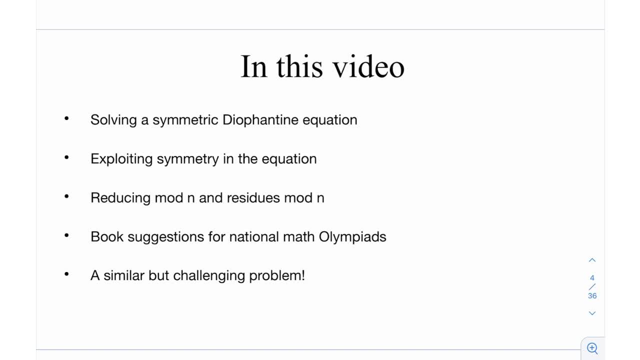 diaphant N equation how we can explore the symmetry given the equation, basically to kind of reduce the R workings And, of course, reducing modern and residues, modern, which is a very critical topic, And after that we will send a book to you. So let's get started. 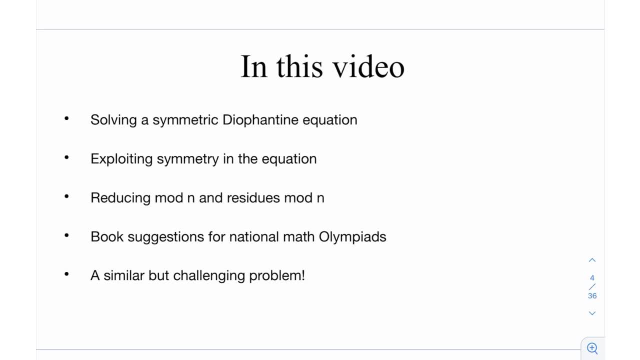 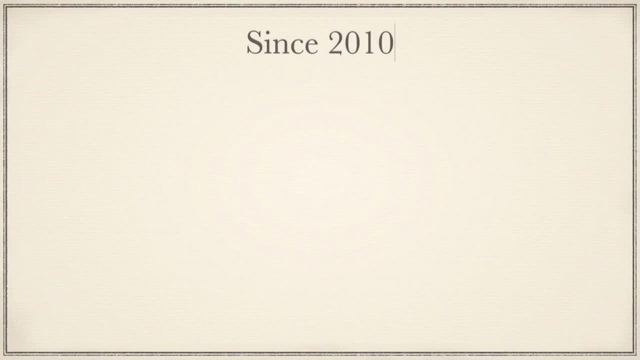 This video is sponsored by Chintacom. Since 2010,, Chinta has trained thousands of students from all around the world in mathematical Olympiads, physics Olympiads, computer science and informatics Olympiads, ISICMI entrances and research projects for school and college students. 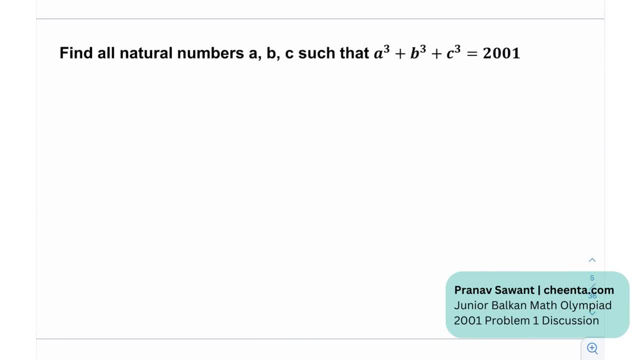 So, yeah, we need to find all natural numbers, ABC, so that AQ plus BQ plus CQ is 2001.. Now, you might have seen this problem before, but we're going to try and solve it in the most efficient way possible, because there are a lot of ways to do this right. But you're. 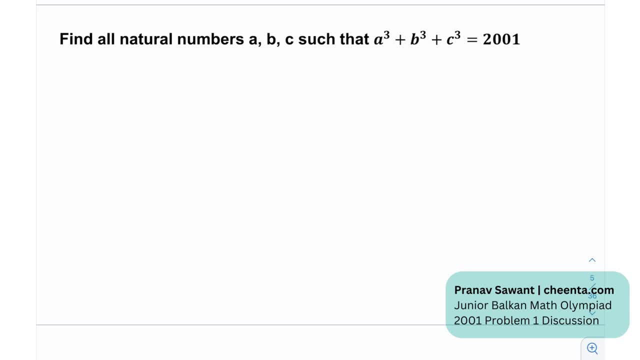 going to try and use as many number theory toolkits that we might have in order to, you know, get through this Right. So what do I see? So, first, I see that the equation is symmetric. you know, replace A with B, B with C and C with A, The equation is still the. 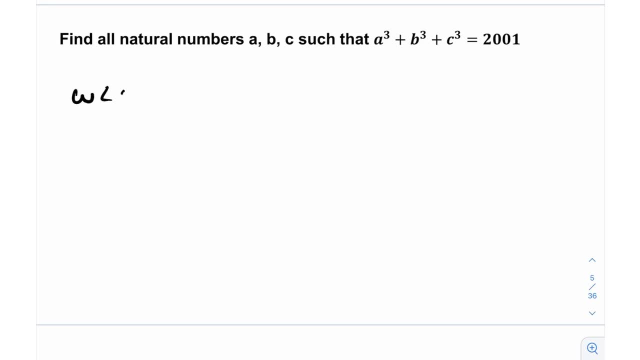 same Right. That's great, because then I can write without loss of generality. I can assume A greater than, equal to B, greater than or equal to C, due to symmetry, of course, Right, And one of the many reasons why we do this is: 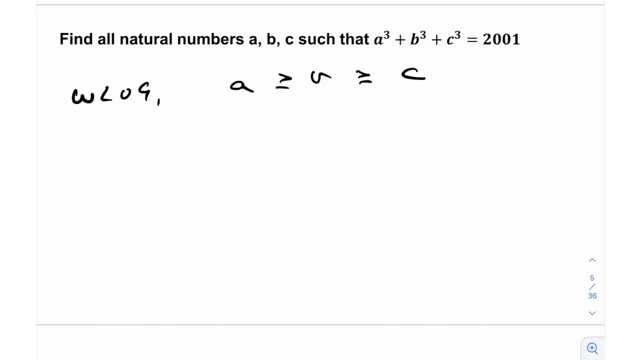 to kind of get this AQ plus BQ plus CQ in a certain bound, kind of bounded to two intervals in a way. So for example, AQ plus BQ plus CQ would then be less than or equal to AQ plus AQ plus AQ. The reason for that is BQ will be less than or equal to AQ plus AQ. 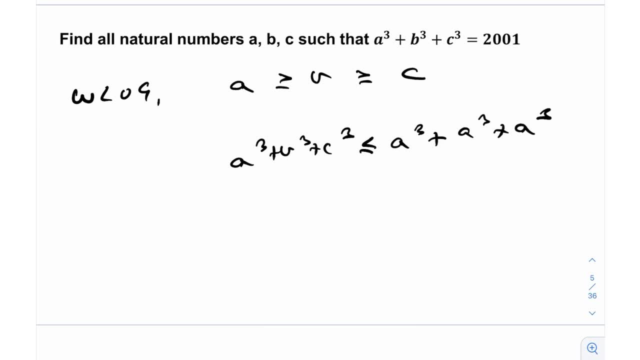 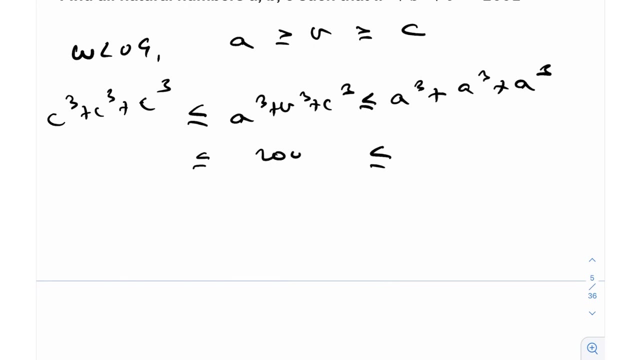 And same with CQ as well, But at the same time, this will be greater than or equal to CQ plus CQ plus CQ, because C is the smallest of three And, similarly, A is the largest of the three. OK, so this AQ plus BQ plus CQ, which is 2001,, is bounded between two. 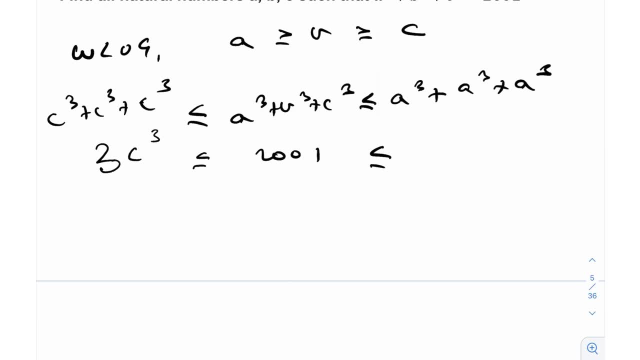 values. It's bounded between two CQ, three CQ brother and three AQ, And it just so happens, It just so happens that 2001, divided by three, happens to be an integer. So that's what we're going to do: We're going to divide by three. We're going to divide by three. 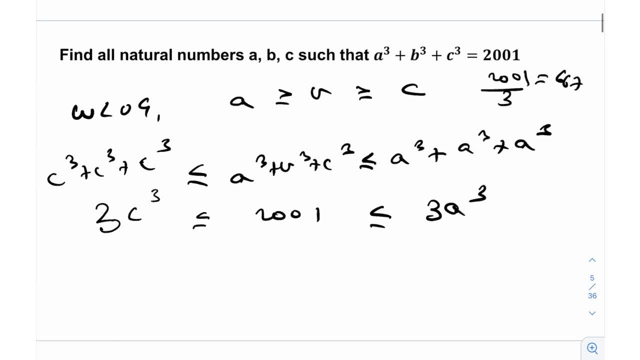 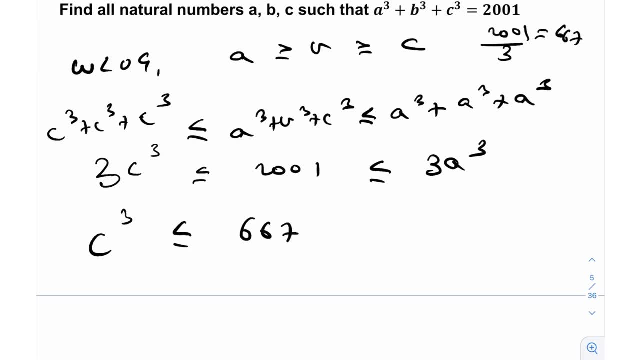 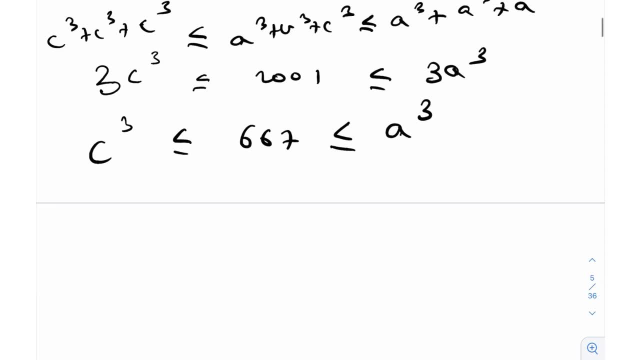 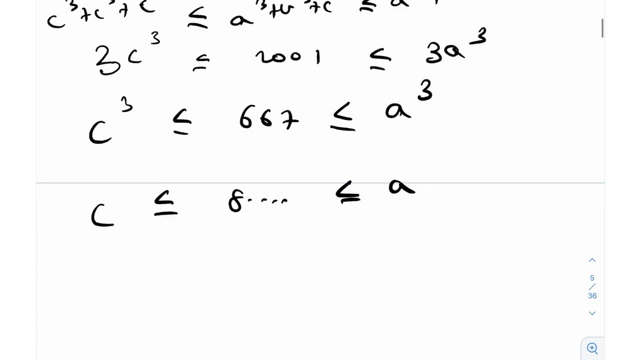 equal to AQ. Now, if we just take the cube root on both sides, I'll get cube root of 667, which is eight point, something which is less than or equal to A. So from here I can make the conclusion that C is less than or equal to 8 and A needs to be greater than. 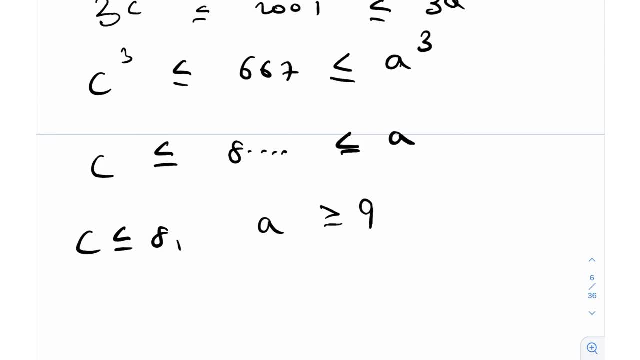 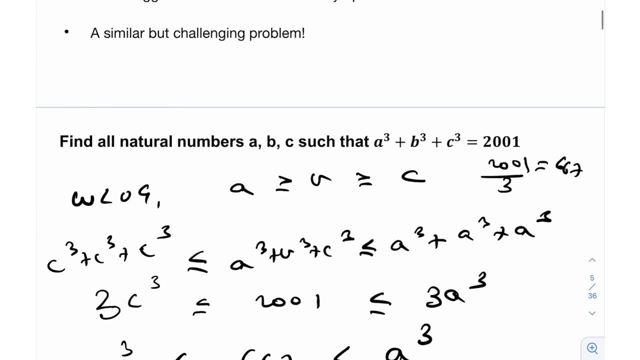 or equal to 9.. OK, this is awesome. okay, this is awesome because now you've, in a way, limited the values of c. c can only be one to eight. right, because it's a natural number, a, b, c need to be natural numbers, right, natural numbers. 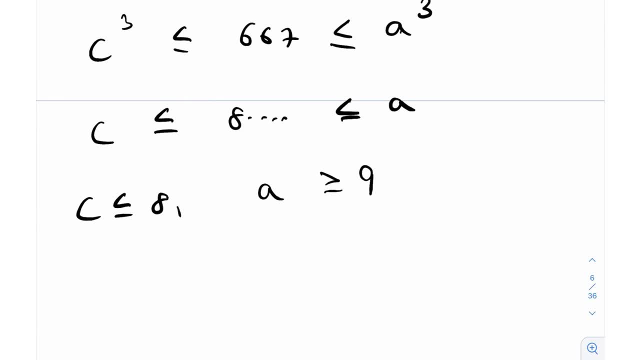 so c can only be one to eight, so you can proceed with making cases, a very inefficient method, let me just tell that as well. so we're going to try and maybe simplify our work further, right, instead of making cases, because who likes making cases, right? so, like, just look at here, what have we done? 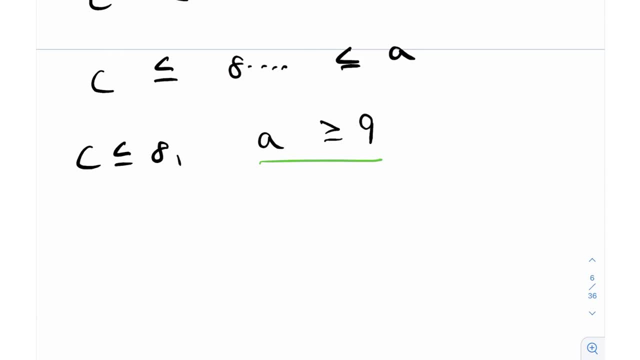 we found out the minimum value of a. so if i ask the question: what is a max can? can there exist a maximum value of a? and the answer is yes. so if you just look at the equation, a cube plus b cube plus c cube is equal to 2001. now if i just tell you a, b and c can be anything. it can be any real numbers. 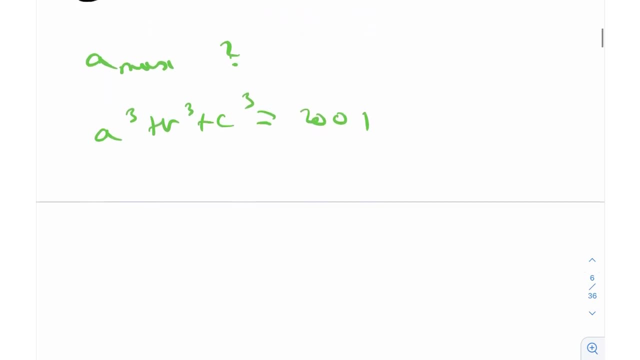 positive real numbers, right, including zero. then you would say that, well, the maximum of a would occur when b and c are zero. right? so, using a similar idea, a q plus zero plus zero would be less than or equal to 2001. right, so a cube is less than equal to 2001. 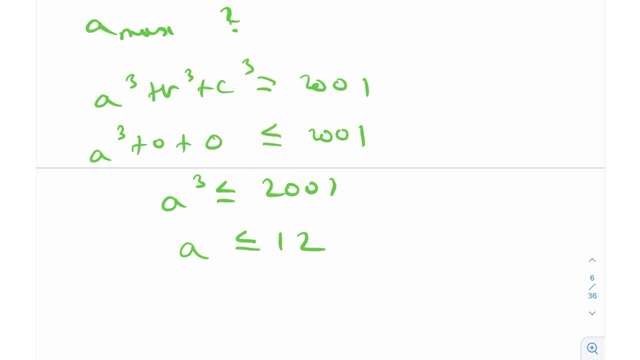 and if i take the cube root i can get: a is less than equal to 12. it's amazing because from this and this, i can really bound the values of a between two- two like numbers, right. so a is between 9 and 12. and we have also another result: c is less than or equal to 8. now this is amazing. 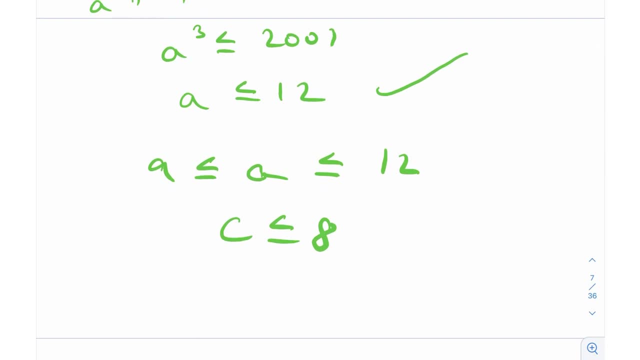 but this is again shortened down our work. now you can do casework a, 9, 10, 11 and 12. you need to only check for four cases and obviously solving a diaphragm- 10 in two variables is significantly easier. right, so you can go with casework at this point, which would 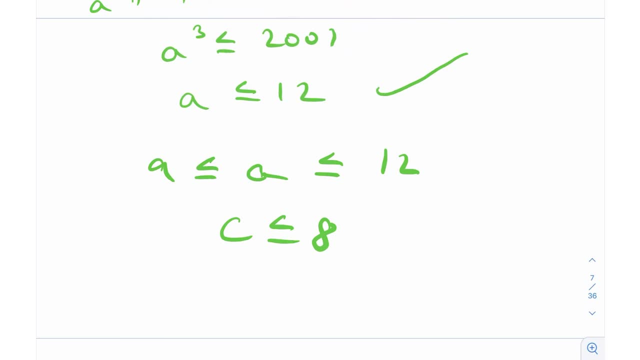 still be a brute force method, because there does exist slight more simplification to this, and that is using the concept of um, modular right, modular residues. how can we use that over here? well, here's a tip. whenever we have cubes, it's very easy to use mod 9, and there's a reason for that. i'll 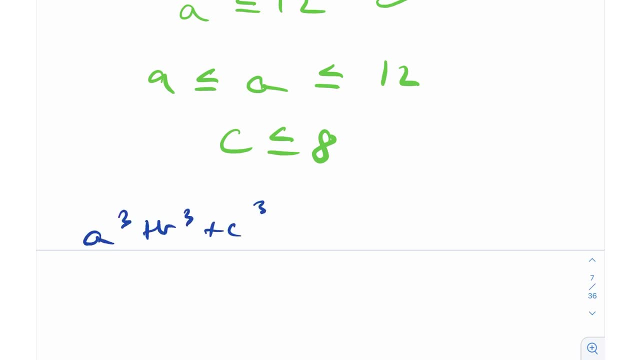 explain you how. so we have a cube plus b cube plus c cube is equal to 2009, 2000 and, uh, 2001. so happens to be three mod 9, right? okay, that's great. so we tend to reduce mod 9. basically, that's the. 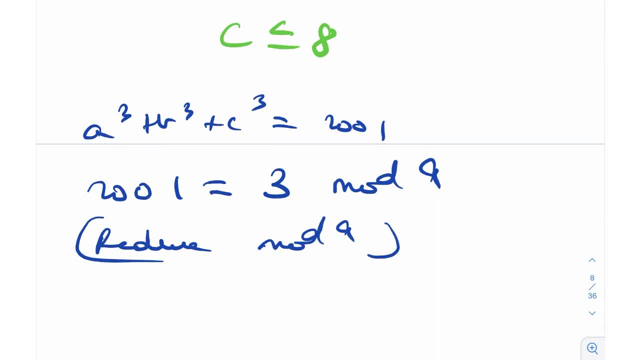 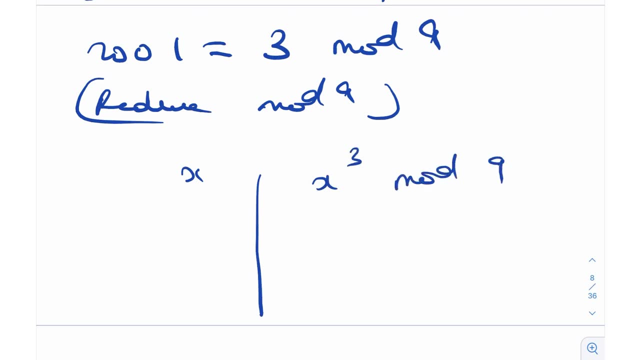 idea: reduce mod 9. that's the idea, that's the key idea over here. so if i just kind of notice the residues that we get of cubic residues, modulo 9, so for example, if x is 0, 0 cube mod 9 is 0, if x is. 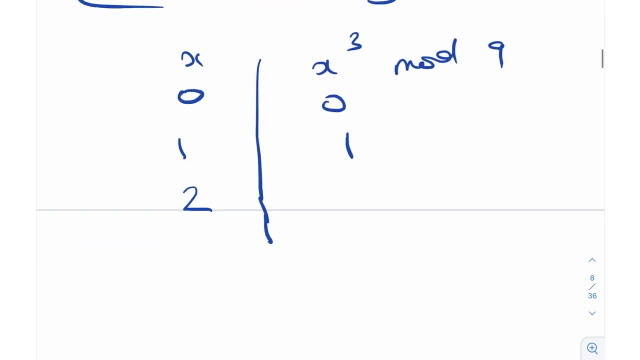 1, 1 cube mod 9 is 1. if x is 2, 2 cube mod 9, 8 mod 9 is minus 1. if x is 3, that is 27 mod 9, 0. x is 4, 64 mod 9 is 1. so if you actually 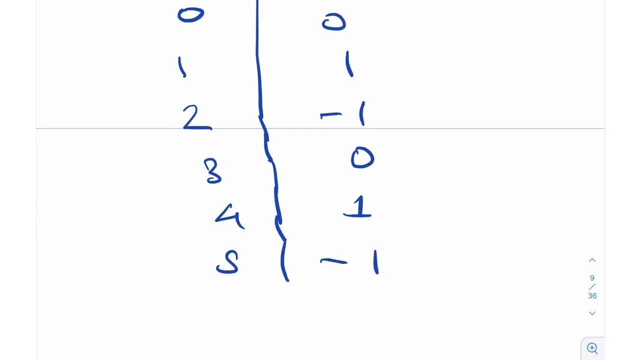 notice this pattern. next will be minus 1, and so on and so forth. so x cube can only be 0, 1 and minus 1 mod 9. that is amazing. so whenever you have cubics, keep in mind that mod 9 can be a good way. 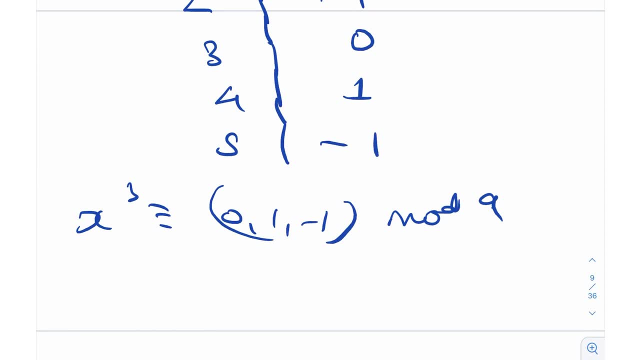 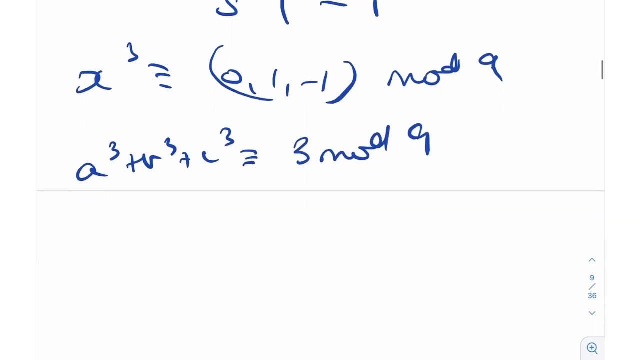 to reduce it down, right, because the cubic residues of mod 9 is 0. 1 and minus 1 is a great really. uh, talk about congruence modulo, right? so now, a cube plus b cube plus c cube, this is basically congruent to 3 mod 9, because 2001 is 3 mod 9. so this can only only only happen if, and only if, 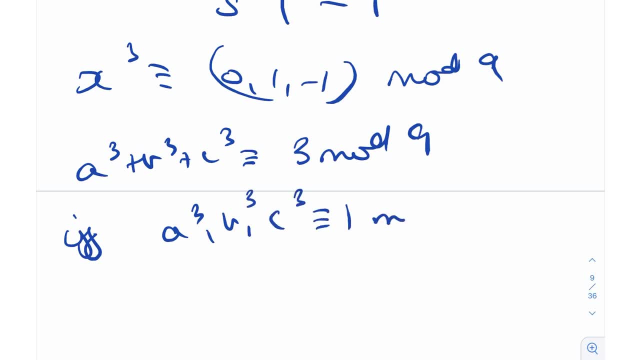 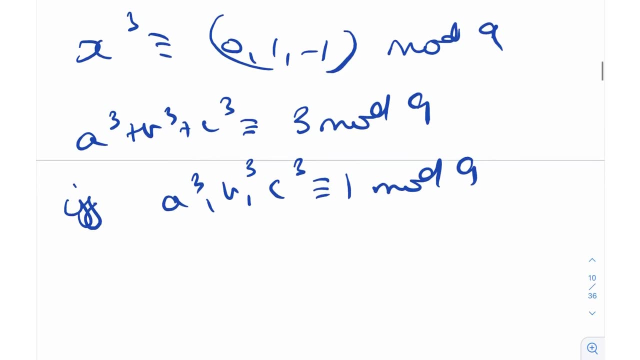 a cube, b cube, c cube are individually 1 mod 9. all of the three need to be 1 mod 9. if there is any other case, then it does not satisfy. right now. i know for a fact that a is between 9 and 12. 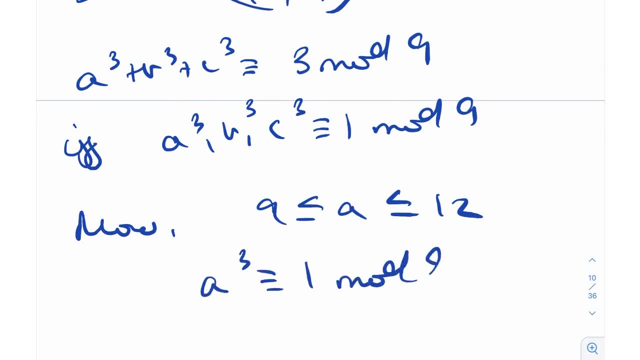 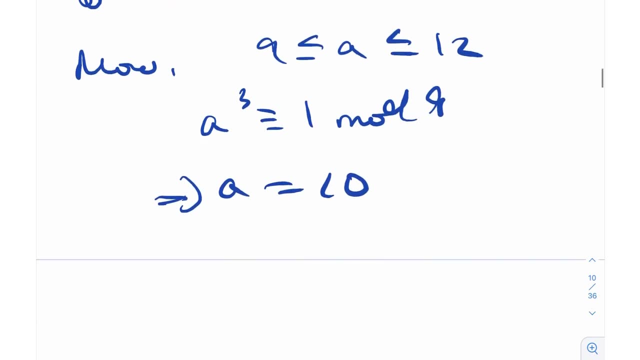 but a cube needs to be 1 mod 9, which implies a has to be 10, because there is no other value of a for which you will get 1 mod 9, right? so a is 10, that's fixed right. so we found out the value of. 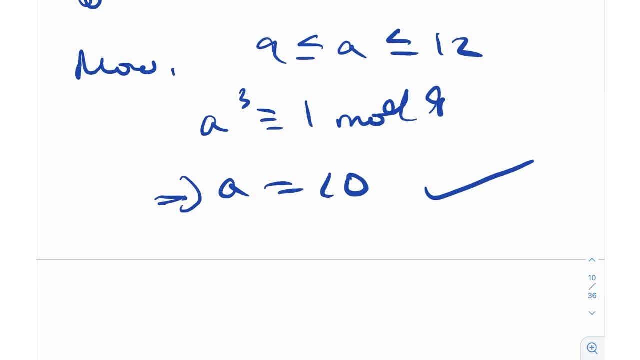 a without really any casework, right, without really any case. we just have to reduce mod 9, so we have the equation: a cube plus b cube plus c cube is equal to 2001. if i just plug in: a is equal to 10. over here i'll get: b cube plus c cube is equal to one double zero one, that's. 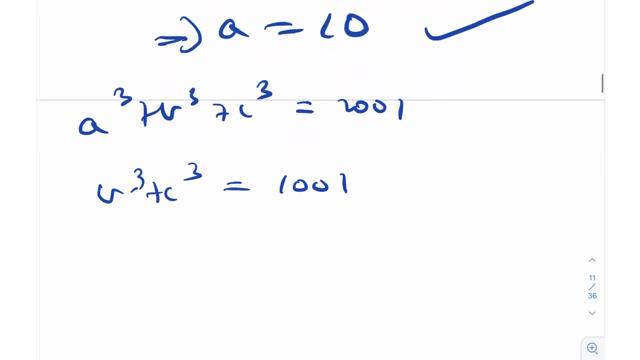 awesome now because you've kind of reduced it down to two variables. the method is still the same, right, without loss of generality. b is greater than equal to c, which is what we'd assumed earlier as well. so, similarly, b cube plus c cube is greater than or equal to b cube plus b cube. 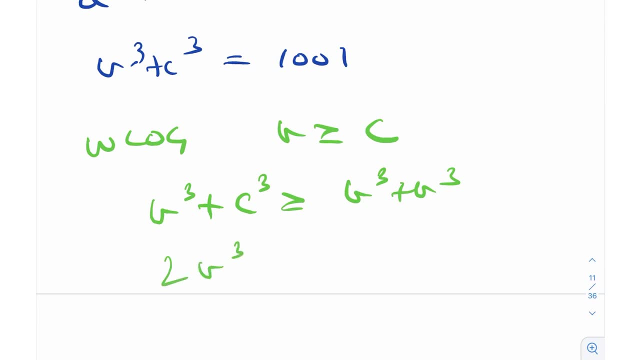 right? so in a way, 2b cube is- or i should write it like this: b cube plus c cube is less than or equal to b cube plus b cube. right, because b is greater than or equal to c. that's the order that we are following, right? or in other words, c is less than or equal to b. okay, great, so 1001 is. 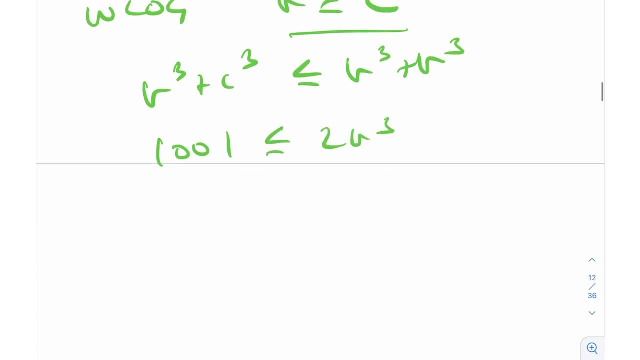 less than equal to 2b cube. right, in other words, 2b cube is greater than or equal to one double zero one. so this gives, in a way, a minimum value of b. now again i asked myself the question: what is b max? what is b max and how do you figure that out? again, just a similar strategy: b cube plus c. 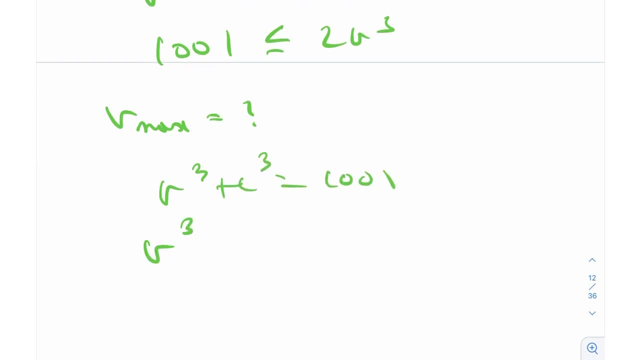 is one double zero, one b maximum will happen when c is equal to zero, just kind of fusing that idea. so b cube is less than or equal to 1001. so b cube is needs to be less than equal to 1001. using this and this, we get a very cool equation, an inequality, rather we get a bound for 1001 in terms of this. 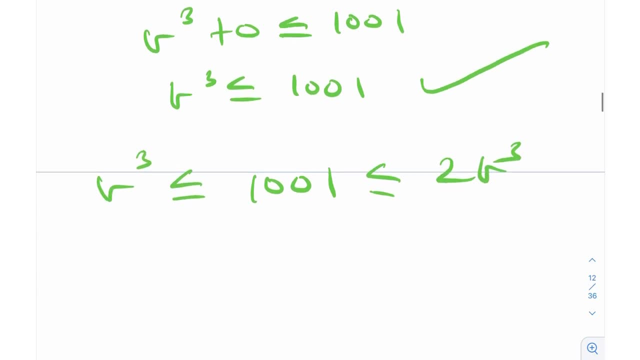 thing b right now. let's solve this. so b cube is basically less than 1001, which implies that b needs to be less than equal to 10. similarly, b cube needs to be greater than equal to 1001 by 2, or in other words, b needs to be greater than or equal to 8. 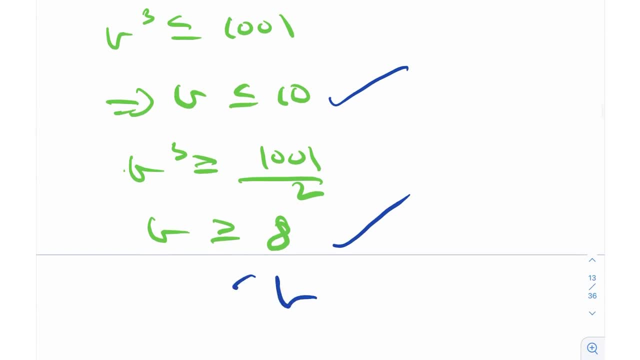 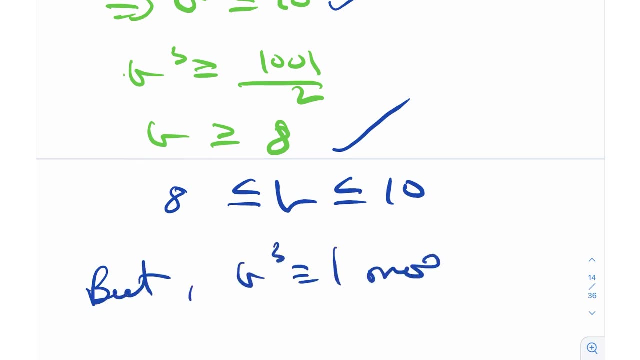 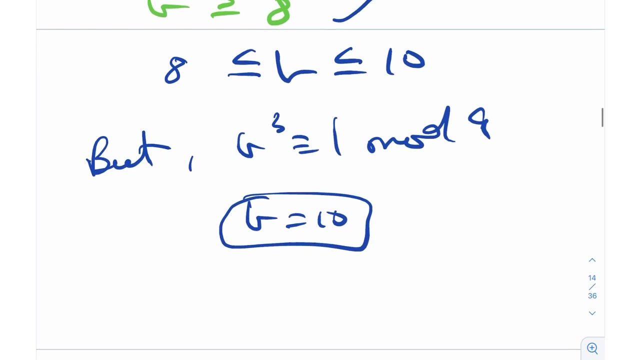 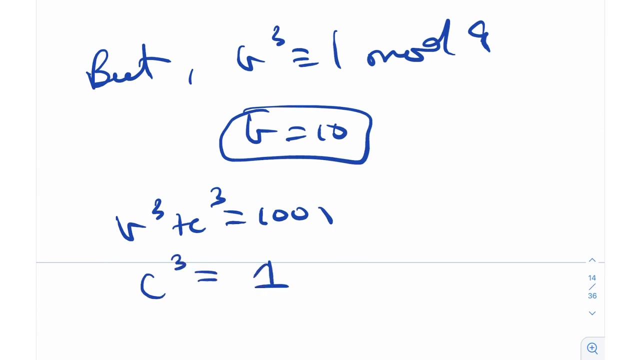 so now again, using this and this, b is also bounded between 8 and 10, but b cube needs to be 1 more 9, right, and the only case for that is when b is equal to 10, so we found another solution as well. now then b cube plus c cube was 1001. so c cube is what it's, just one, or because c is a natural. 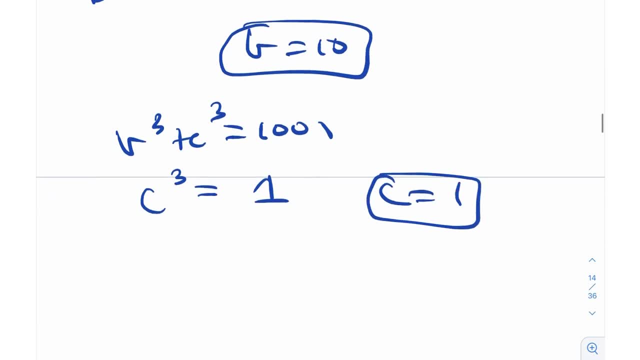 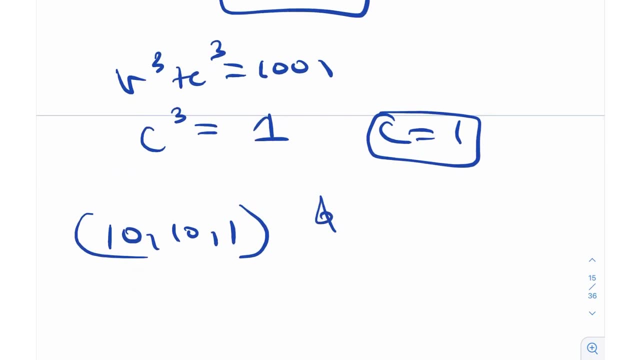 number c then has to be one. so what should be the solution? 10 10, 1. but is that it? no, we write 10 10, 1 and all its permutations. right, because it's symmetrical. if a, comma b, comma c is a solution, all permutations of a, comma, b, comma c. 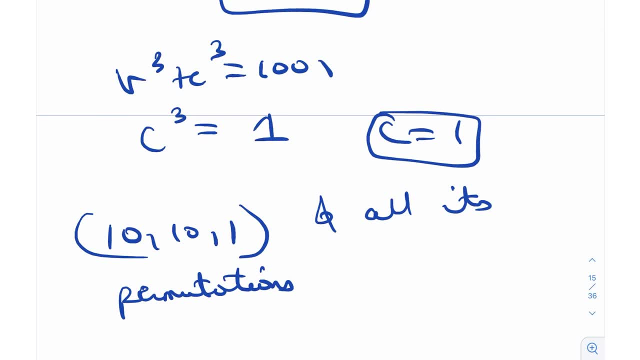 will also be solutions, and the reason why we got only one solution is we- we kind of use the without loss of generality- that a needs to be greater than or equal to b, greater than or equal to c. right, but if you consider some other order, you'll get a different set of solutions. 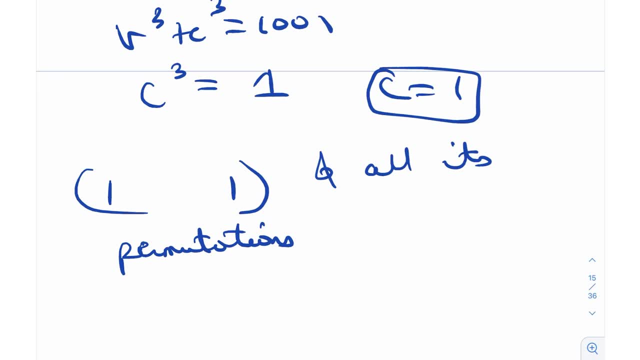 right. so basically 10 comma 10 comma 1 and all its permutations. so for example, 1 comma 10 comma 10. you know, 10 comma 1 comma 10. all of these things will be included in the solution set and that will be your entire solution set. so i hope you enjoyed that. it was, i think, one of the most classic number. 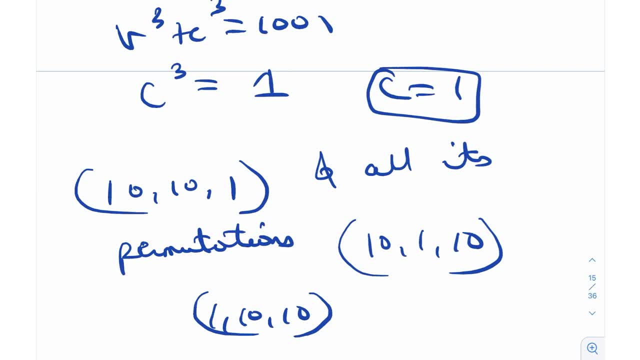 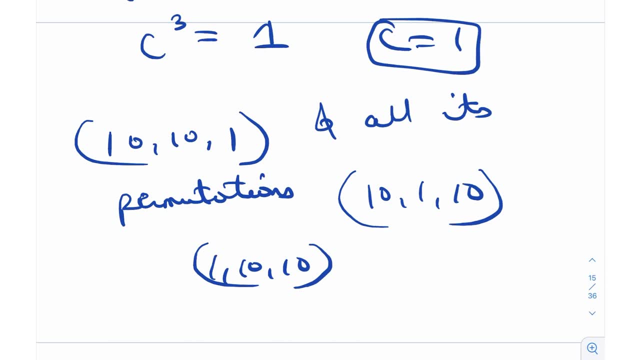 theory problems out there, and this is something that you should keep in mind, especially the fact that whenever you have cubes, mod 9 is a very good idea, right. you can use some other, reduce some other mod n as well, but mod 9 is a very good idea, right? so i hope you enjoyed that and i hope you.